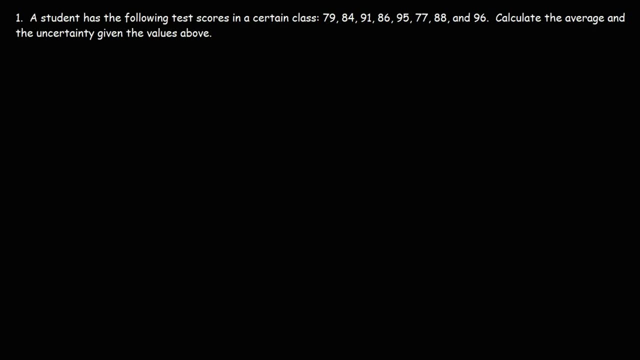 In this video we're going to talk about how to calculate not only the average given a data set, but also the uncertainty in the average. So let's work on this problem. A student has the following test scores in a certain class: 79,, 84,, 91,, 86,, 95,, 77,, 88, and 96. And we need to calculate the average and the. 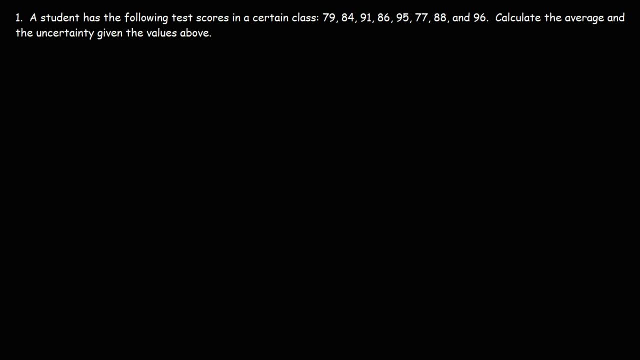 uncertainty in those values. So let's start with the average. The average, or the mean, is going to be the sum of those numbers divided by the number of numbers in that set. So the sum is going to be 79 plus 84 plus 91 plus 86, and so forth. 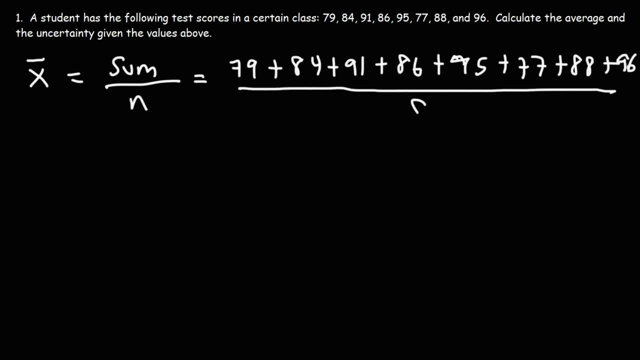 And we have 8 numbers in this list. So the sum is 696.. Now, if we take 696 and divide it by 8, it's going to give us 87.. So that is the average test score. Now, before we calculate the uncertainty, let's talk about the formula, Let's draw a. 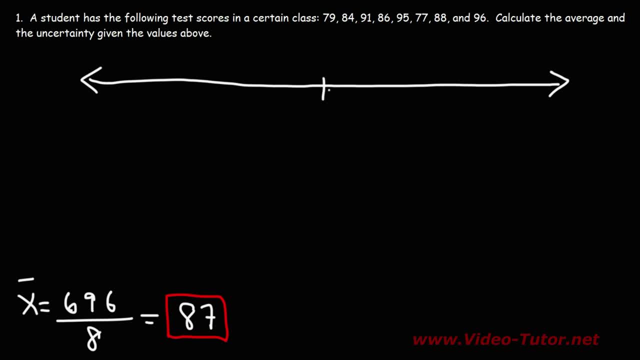 number line. In the middle of the number line we're going to put the mean. The mean is 87.. The highest number in this list is 96.. The lowest number we could see is 77. But within any range, what we have is the upper limit of the uncertainty which we'll 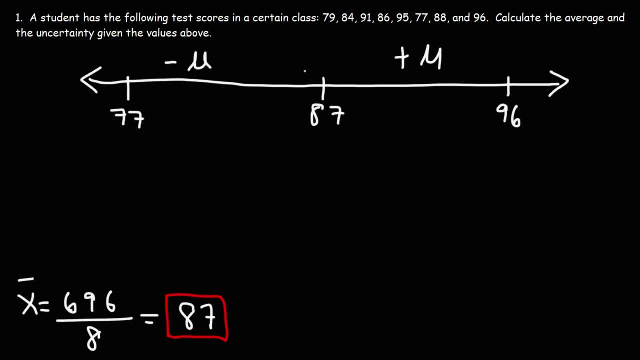 call u and the lower limit of the uncertainty, Let's call it negative u. So if we add the mean and the upper uncertainty, it will give us the top number, And the mean with the lower uncertainty should give us the lower part of the range. So notice, this is the range. 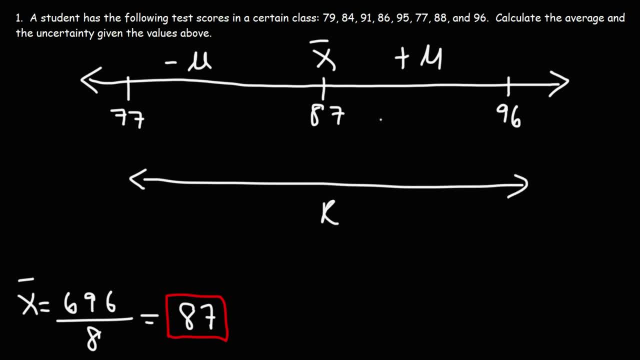 here, The upper half is one half of the range. The lower half is negative one half of the range, which makes sense. It's half of this entire range here. So that's how you can calculate the uncertainty. The uncertainty is basically just one half. 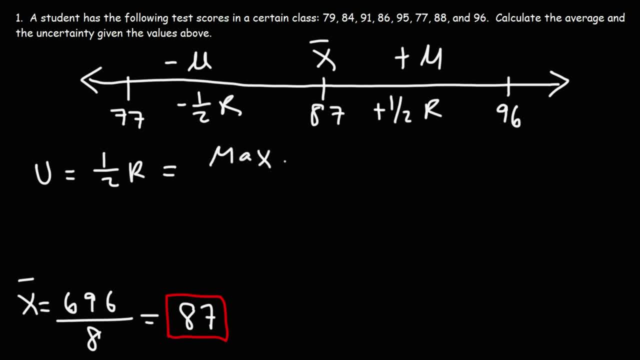 the range. The range is the difference between the maximum value and the minimum value divided by 2.. So in this particular example, our max is 96.. Our min is 77. So we have 96 minus 77, and then we're. 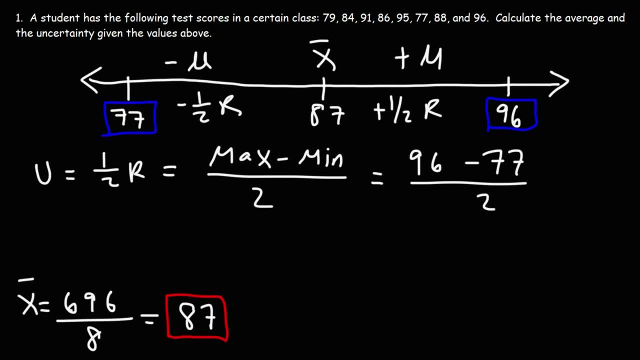 going to divide that by 2.. 96 minus 77,, that's 19.. 19 divided by 2 is 9.5.. So that's the uncertainty in this particular example problem. so now we can write the range of the test scores like this: 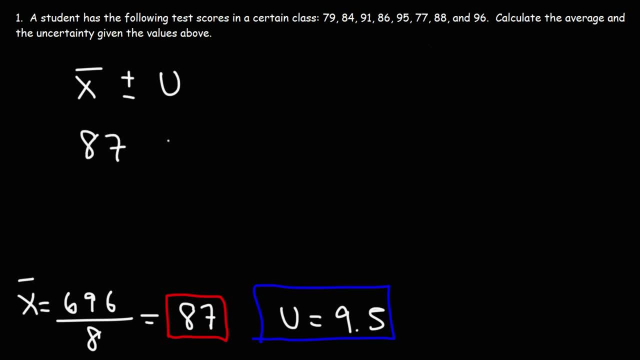 so we have the mean 87 plus or minus our uncertainty, which is 9.5. but typically the uncertainty is usually rounded to one significant figure. so we're going to round it to 10 and so this is going to be our answer. so 87 minus 10 will give us 77. 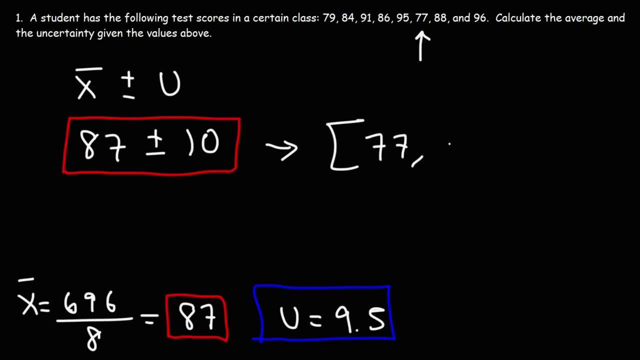 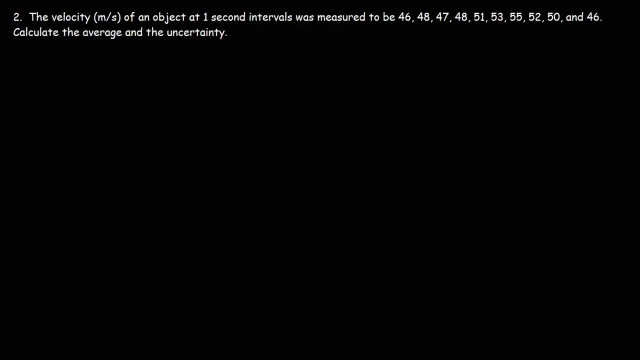 which is the lowest number in the range. 87 plus 10 will go up to 97, which includes the highest number in the range. so all the test scores are in this range. but this is our final answer. this includes the mean with the uncertainty. now, for the sake of practice, 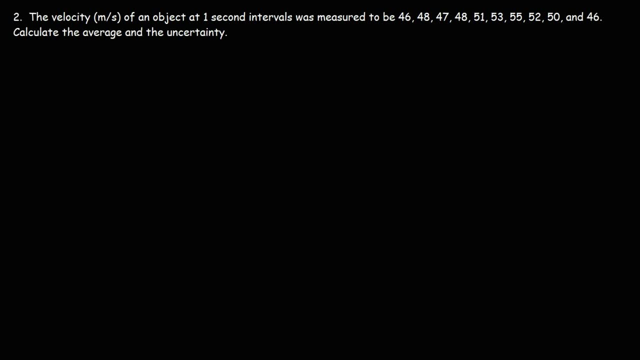 let's work on another example. feel free to pause the video if you want to try this. so we're given values for the velocity of an object at one second intervals. we need to calculate the average and the uncertainty as well. so let's start by calculating the average. 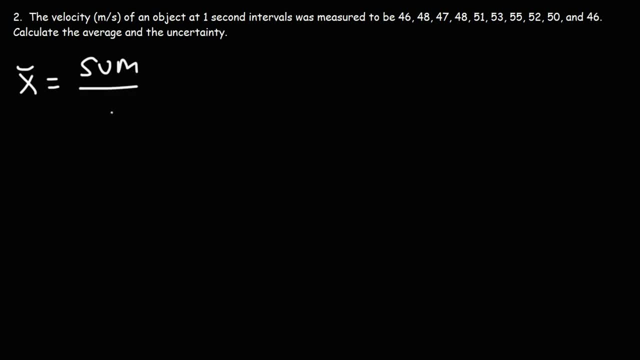 so let's take the sum and divide it by the number of numbers that we have. so we have 46 plus 48, 47, 48 and it looks like we have a total of 10 numbers. so n is 10. now let's plug this in. 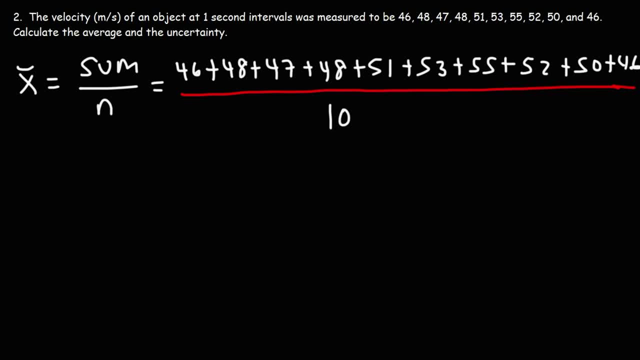 so 46 plus 48 plus 47 plus 48 plus 51 plus 53 plus 55 plus 52 plus 50 plus 46. So I got 496 as a sum, And when we divide that by 10, that's going to be 49.6.. 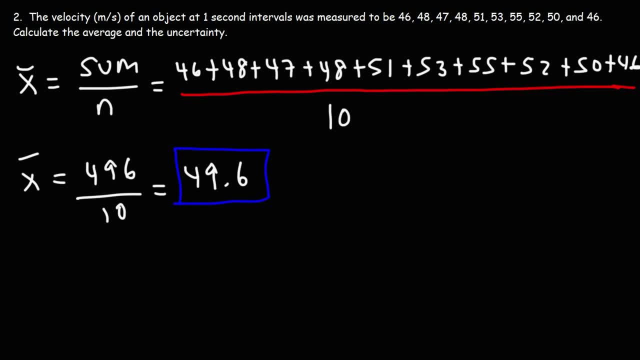 So that's the mean for this problem. Now let's calculate the uncertainty. The uncertainty is one-half the range And the range, the maximum is 55. That's the highest number minus the lowest number. the minimum is 46.. 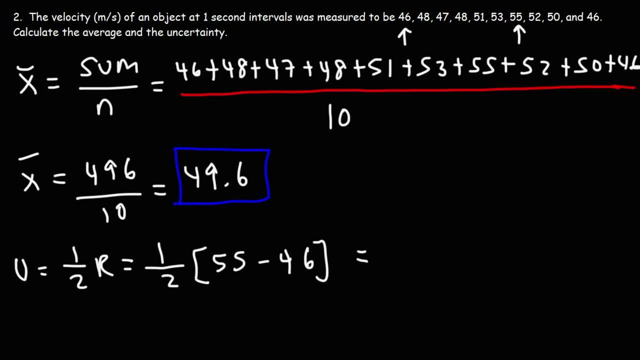 55 minus 46 divided by 2 is 4.5.. And we can round that up to one sig. fig, So we'll say approximately 5.. So the velocity in these 10 seconds we could say it's 49.6 plus or minus 5.. 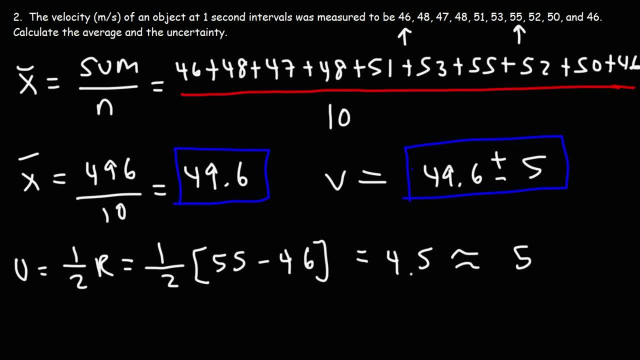 5 is our uncertainty, And let's see how accurate this is. So 49.6 minus 5,, that gives us a lower limit of 44.6.. And 49.6 minus 5,, that gives us a lower limit of 44.6.. 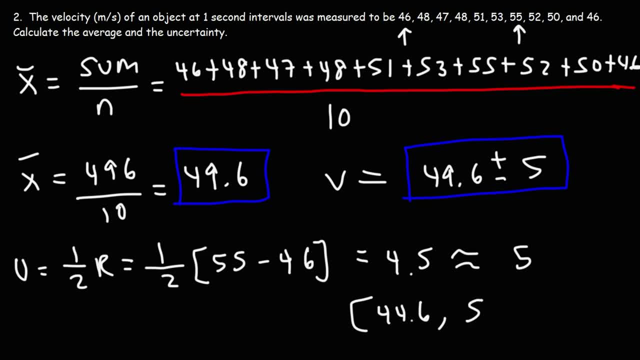 And 49.6 minus 5, that gives us a lower limit of 44.6.. 49.6 plus 5 gives us an upper limit of 54.6.. Now, 55 is just outside of this range here, But nevertheless it's still a relatively accurate representation of this data set. It's not perfect, but it's close to it.